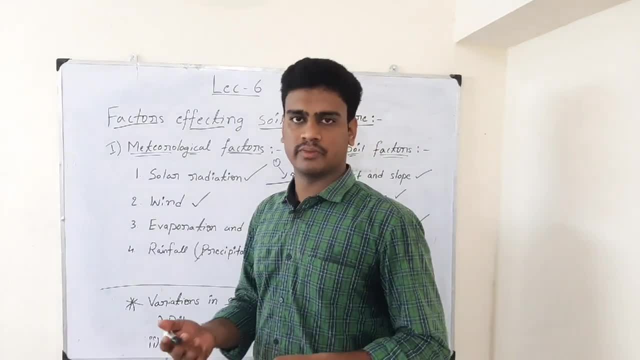 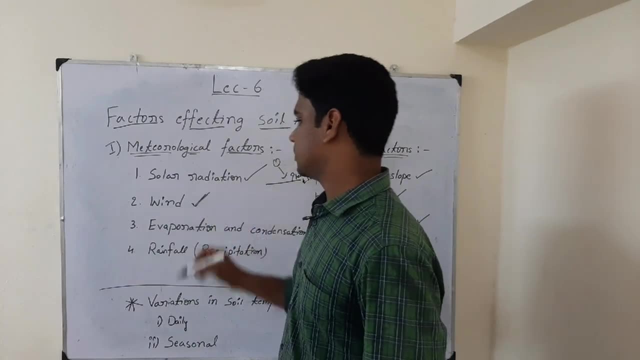 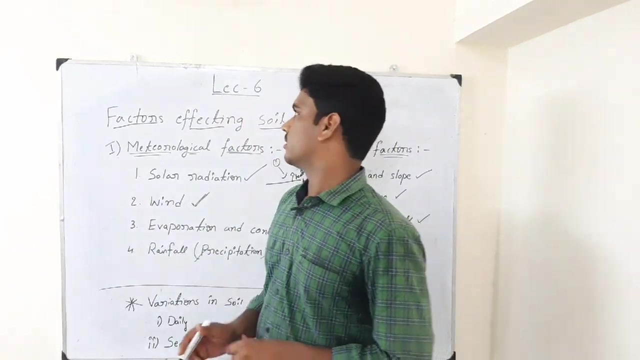 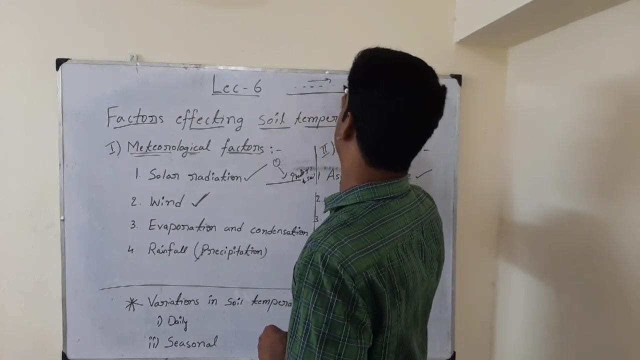 negative way. so the optimum temperature will always help the crop. if it is less, then that it will cause harm to the crop, or more, then that also it may cause harm to the crop. Next one is wind. See, wind is something like air temperature. Wind is something like air temperature only. but now, when this is just imagine, this is surface of the soil. On the surface of the soil, wind is blowing towards one direction and this wind is having some particular temperature. 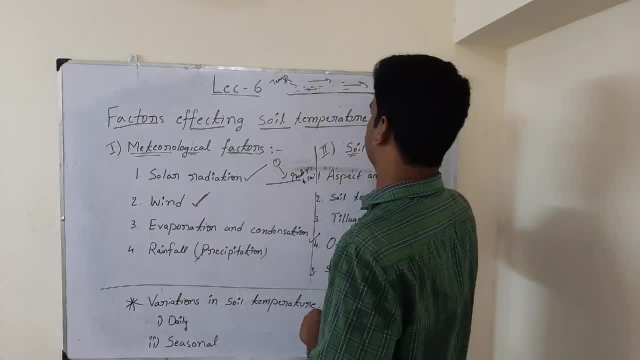 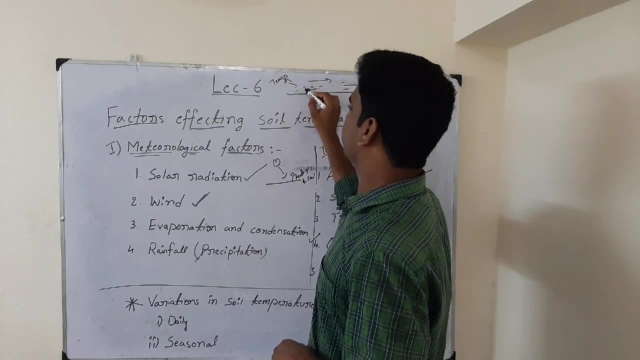 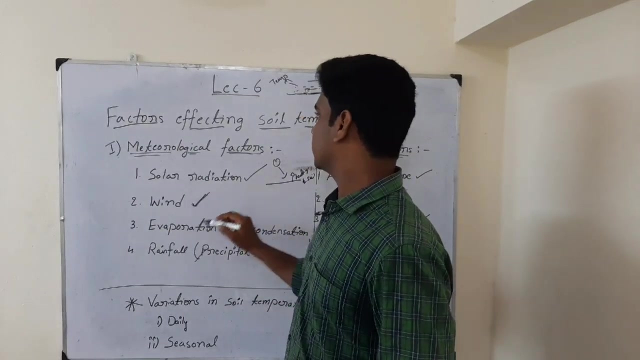 So when this wind is blowing from one place to the other place on particular surface of the soil in that particular location, the temperature which is present in this air will be transferred to that particular soil. So indirectly this wind also is getting affected the soil. So this is about wind factor. 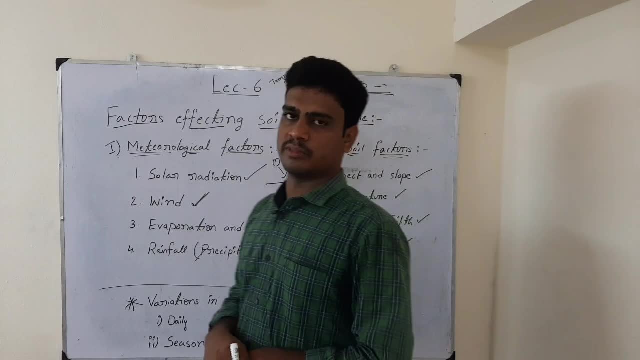 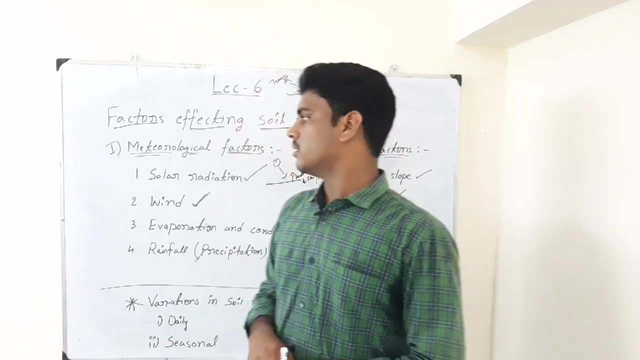 Then next one is evaporation and condensation. You know the meaning of evaporation. Evaporation means loss of water from the surface of the soil, So the soil is called evaporation. So when evaporation after we give. for example, let us take in the cropped field where we are raising the crop. 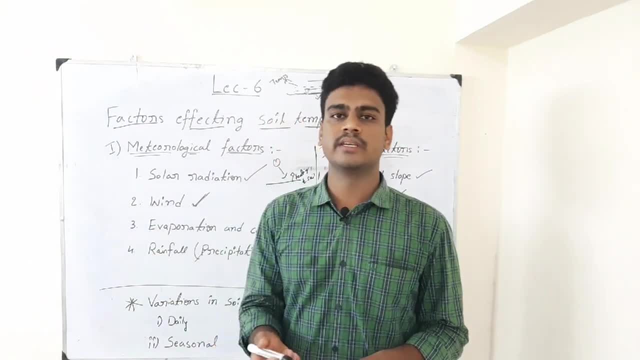 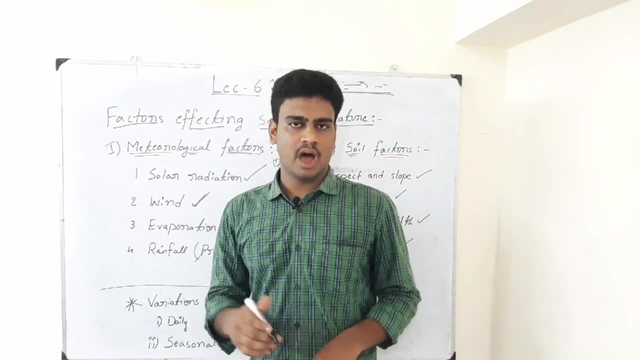 In the cropped field after we give the irrigation, we see evaporation as well as transpiration. Both together we called evapotranspiration. So when we look at the evaporation after big irrigation, immediately some amount of evaporation is taking place from the soil. 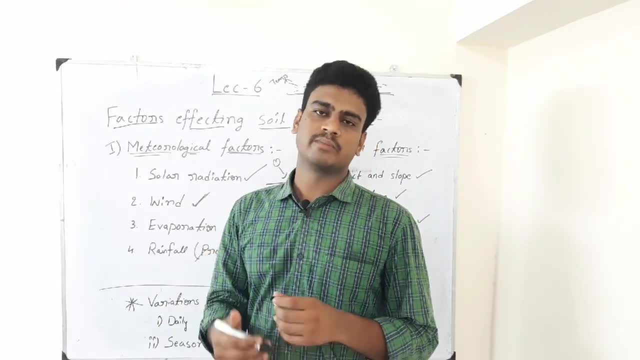 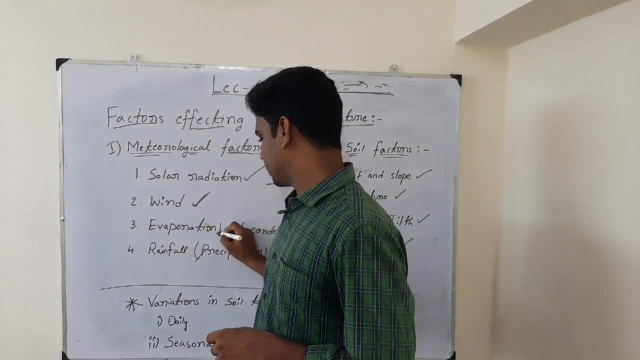 So while evaporation is taking place from the soil, then we can reduce the temperature of the soil. When evaporation happens, the temperature of the soil will get reduced is happening. so temperature of the soil will come down. when evaporation happens, then condensation- hope you know the meaning of condensation. condensation- 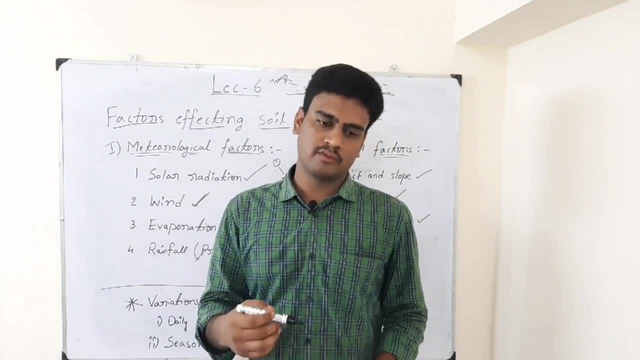 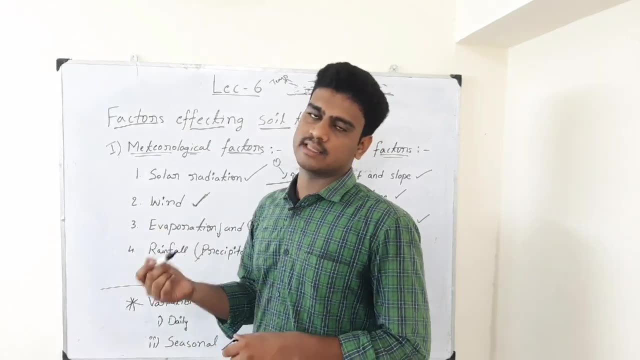 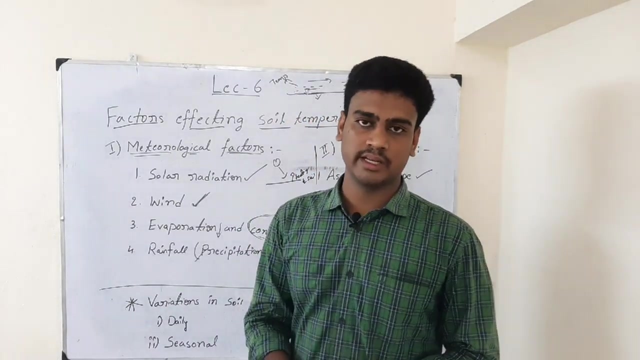 means, instead of going forward, backward. that means turning of water into the vapor instead of that in reverse, vapor is turning back to the water and water turning back to the ice. that we call condensation in condensation. also, when vapor turns back into water in the soil- I am telling inside the soil because of high temperature. till then the water may be turning into the vapor, but because of low temperature or because of no escape of vapor from outside the soil again, that vapor will get stick into the another soil particle and as time passed that those water molecules join together again and they will form again. 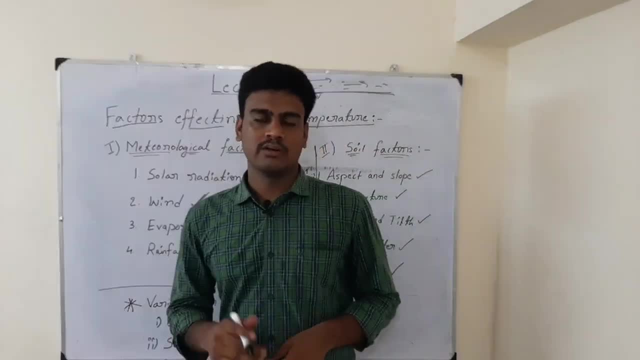 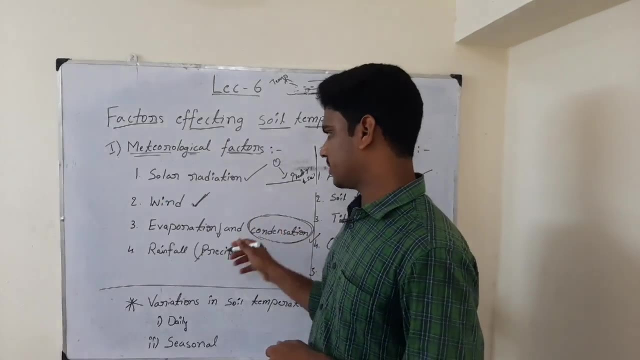 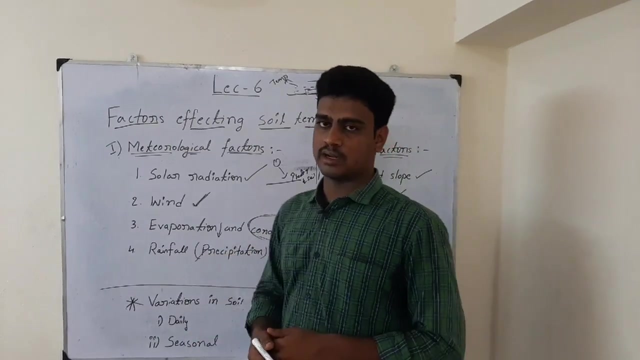 water bag that we call condensation. this is all about when temperature increases, condensation increases. so when temperature increases, condensation will happen in the soil- soil. then next one is rainfall. the other name of rainfall is precipitation. I'll explain when that particular topic comes. what's the difference between the? 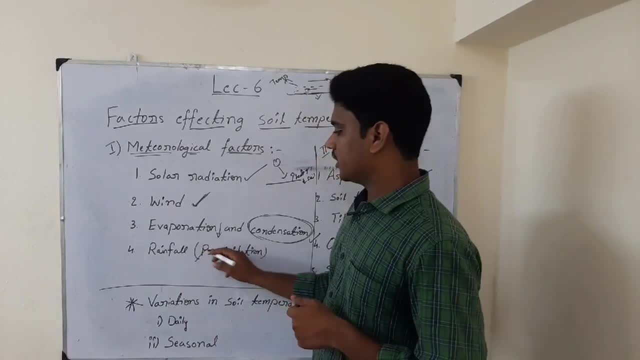 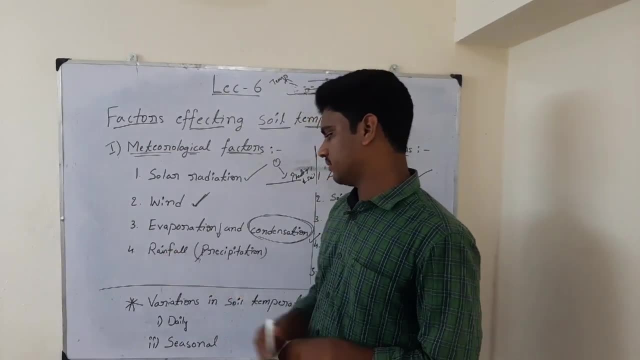 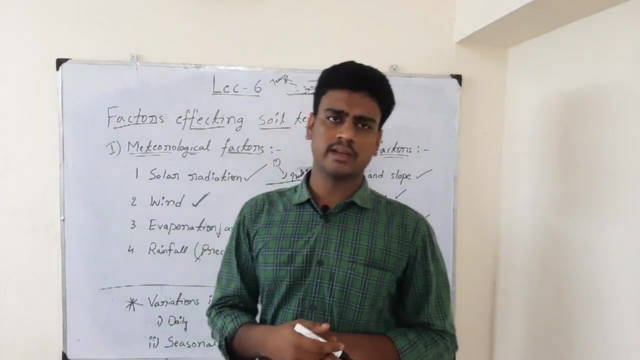 precipitation and rainfall. so actually we call precipitation for all the in the, in the precipitation only the, subdivided into different types. so among the world, among them, one is rainfall. so you all know the meaning of rainfall. so, based on the water droplet, it will be so when that particular rain droplet or water. 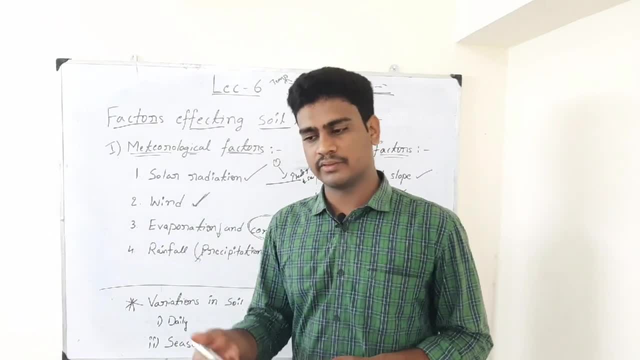 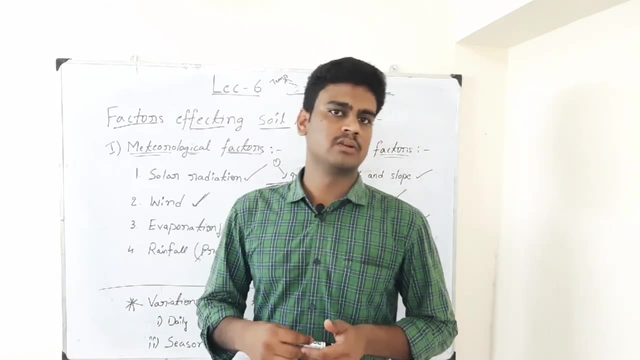 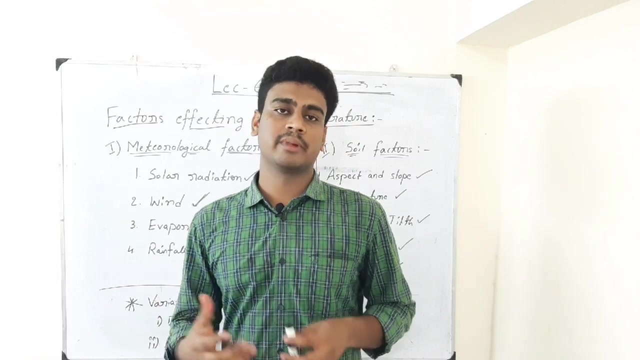 droplet is having the particular temperature, the same temperature when it falls on the soil. soil temperature also will get affected because most of the rains will be cool. but during the summer season in the warm climate regions the rain droplet temperature may be varied. it may be little warm, that warmness which is present in the rain water droplet when 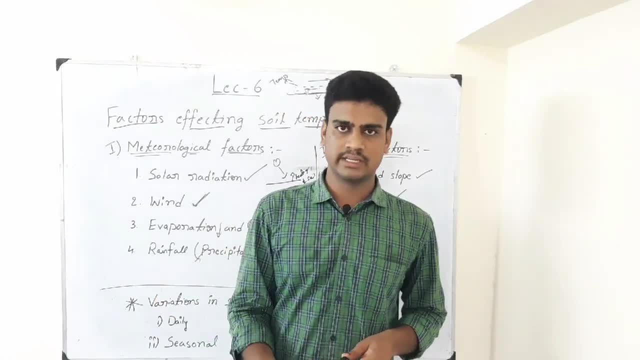 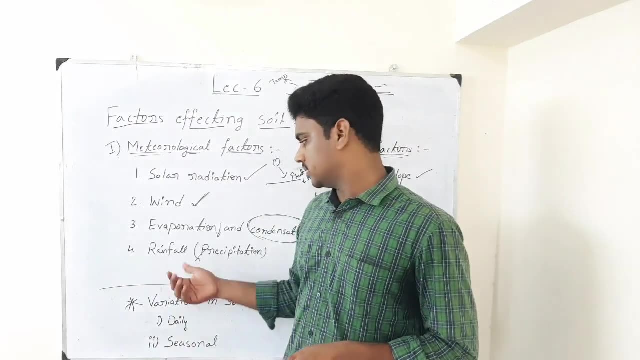 it hits the ground and when it goes into the ground, infiltration. and when it goes into the ground, the soil temperature can be changed. when it falls on the soil, the rain droplet by this rainfall water. So these are the four factors which are affecting the soil. 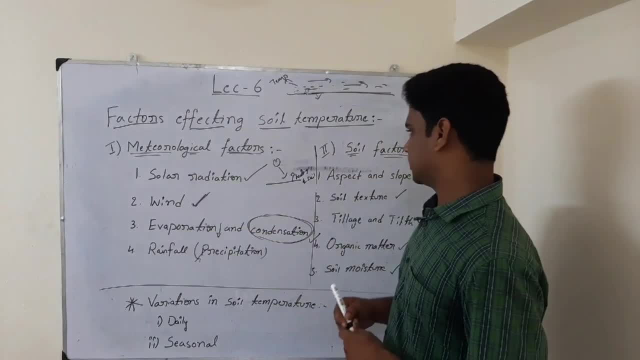 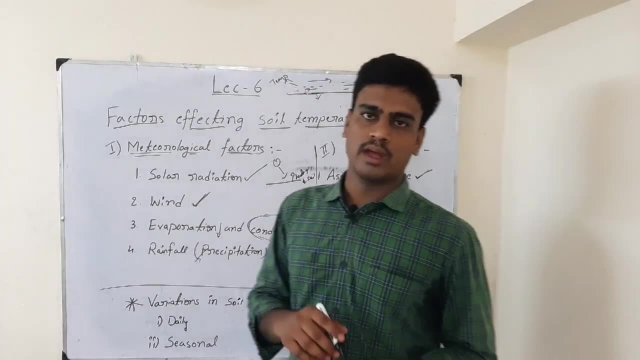 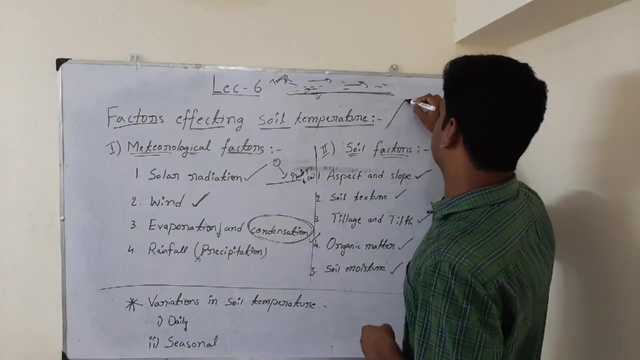 temperature. These all together we call meteorological factors. Next, let us see soil factor. Soil factor: the first one is aspect and slope. Aspect and slope means at what level the slope is, in what angle the slope is, and all. So, for example, let us take the slope may be. 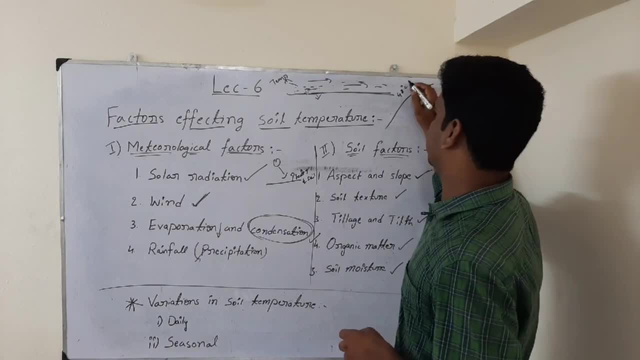 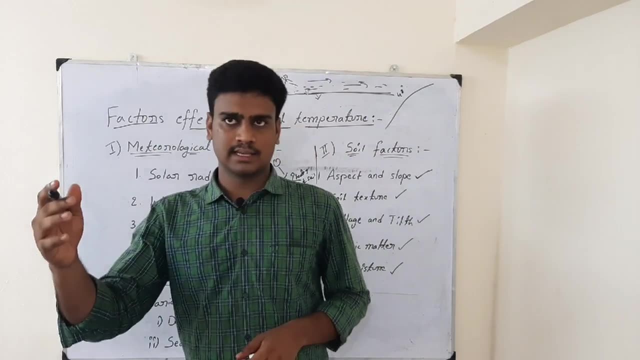 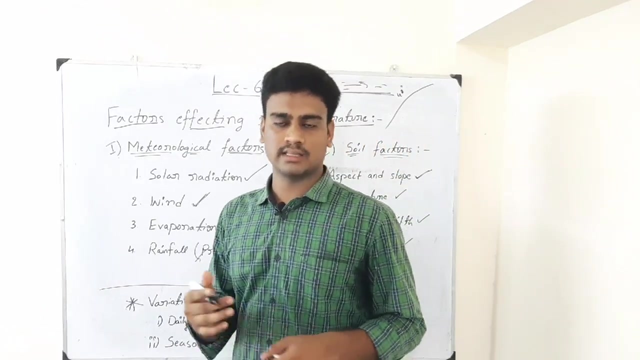 some 40 degrees slant. Let us take example. I am telling 40 degrees slant. So here, when we look at the sun insulation or the sun rays which are striking on the surface of the soil, at what angle are they striking? Are they striking in the southern angle or northern? 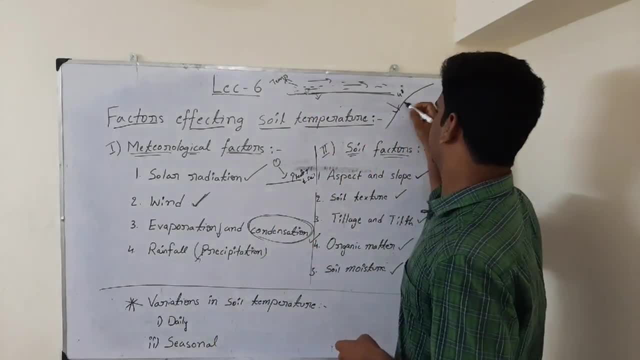 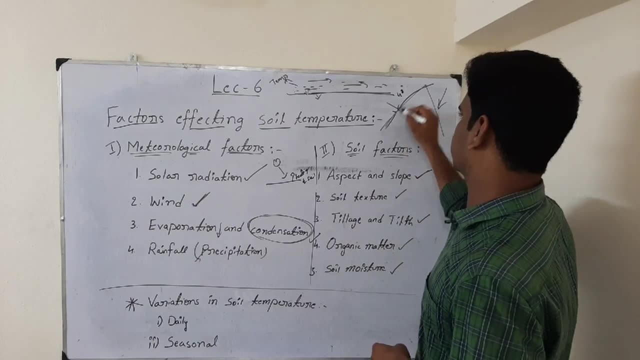 angle. If they are striking to the southern angle, then they are striking into one direction. If they are striking into the northern angle, they will be striking the other side of the mountain. Let us take this as a mountain, and when the sunshine rays are striking one side or one, 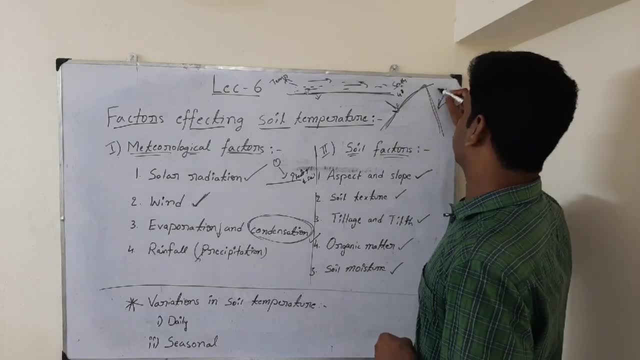 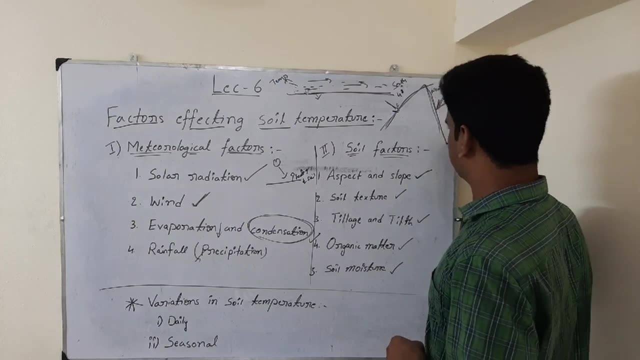 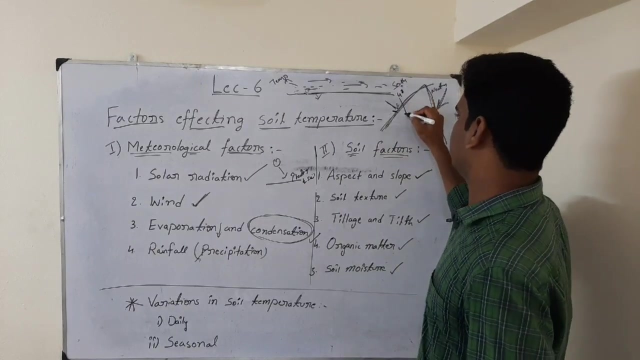 direction. that may be southern side and sometimes sun may strike in northern side. When northern side sun rays are striking this side alone, the temperature of the soil will increase. but the other side sun rays cannot hit, So this side soil temperature will be less. but 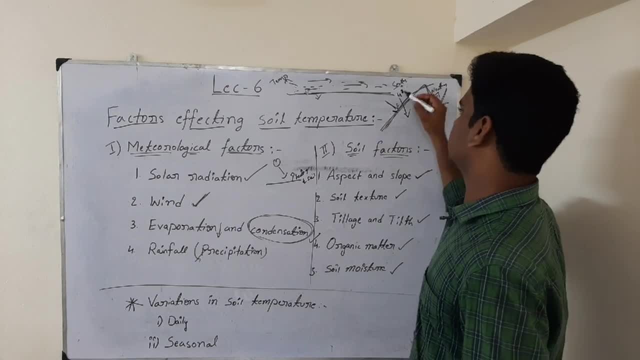 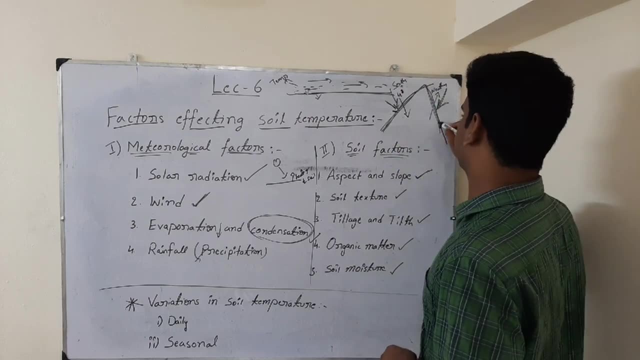 this side soil temperature will be very high In case. in other case, when soil, sun rays hits the mountain, the southern side, then this side temperature will be high and this side temperature will be less, For example, as I am telling, but when we come to the larger 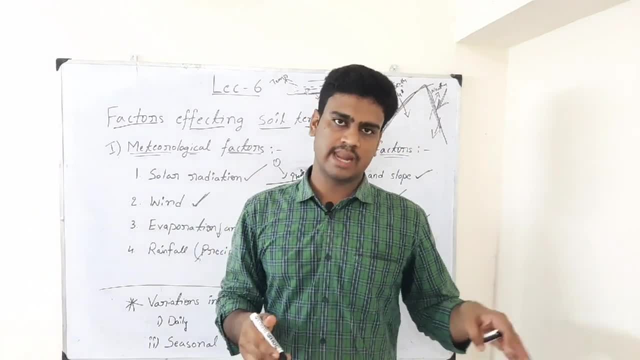 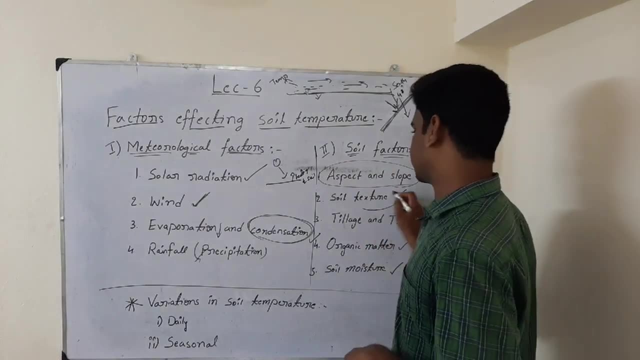 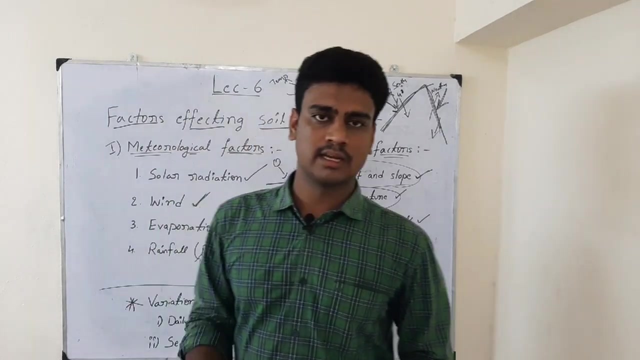 area. it will be varied based on the sunshine comes, the direction and also the slope of the land, and so this is another factor which cause the soil temperature. Then soil texture. In soil texture we see different types of soils. are there Sandy soil, is there clay? 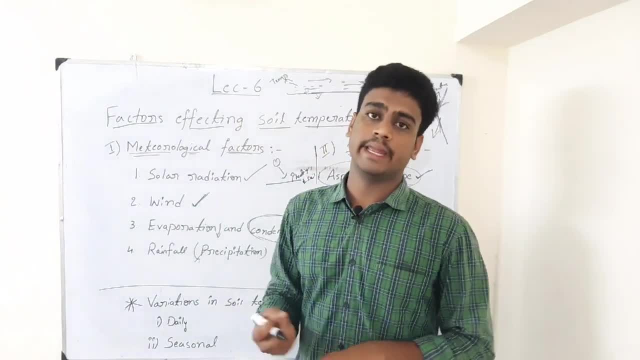 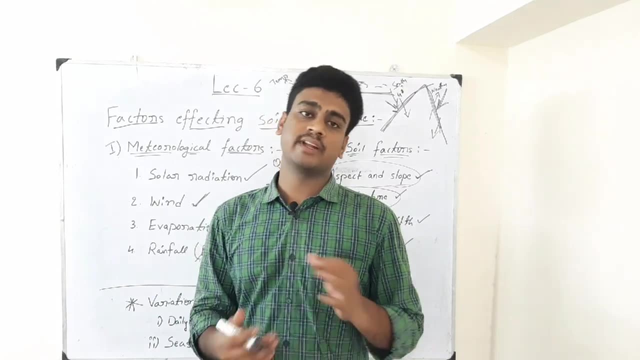 soil is there, silt soil is there. So this is another factor which cause the soil temperature. Then soil texture. In soil texture which soil absorbs more heat. So always remember black body absorbs more heat and light body absorbs less heat. Reflection will be very high in light body. So but when? 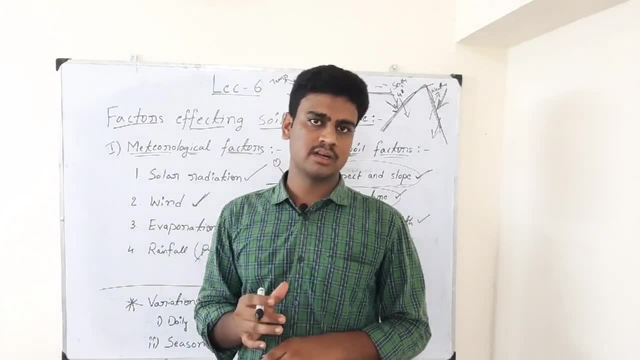 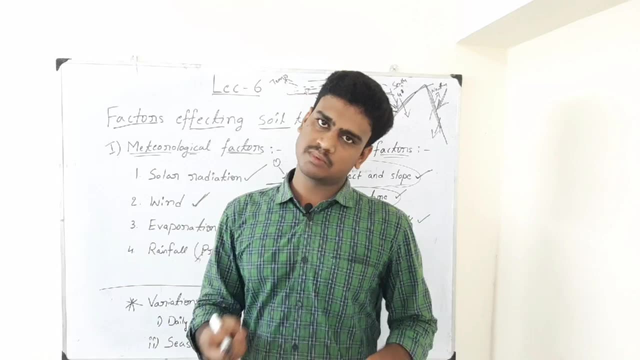 it comes to the temperature in light soils, always remember: light soils heats up very quickly and cools down very quickly. But when it comes to the black soil, black soil absorbs the heat and it cools down very slowly. So that is the difference between the light soil. 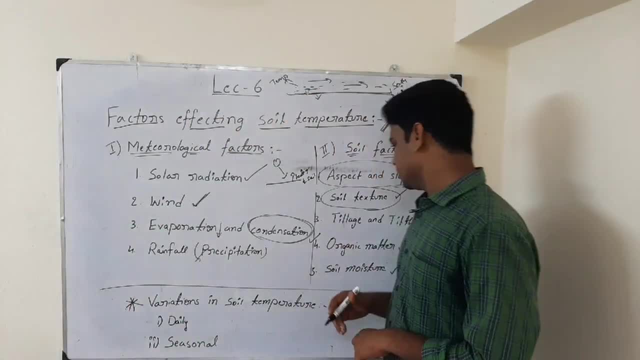 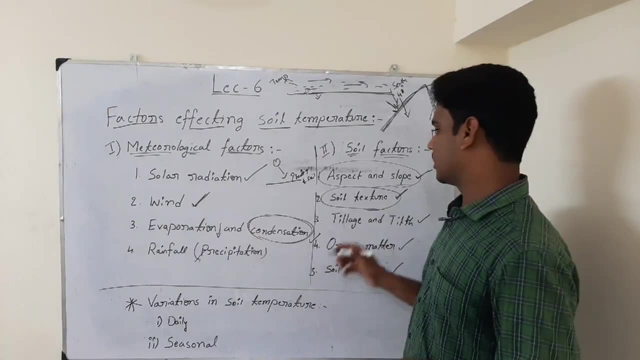 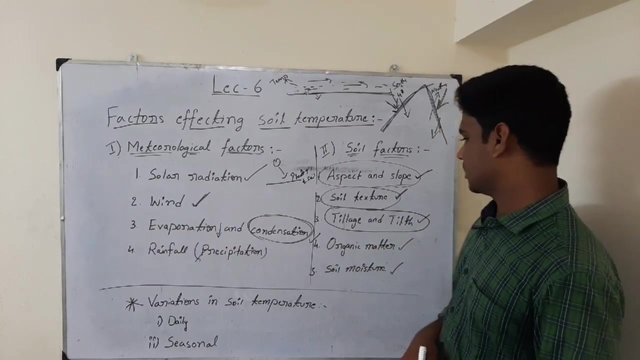 and black soil. So here in soil texture, based on the texture, it will be varied and the color of the texture, I mean the soil, will be varied based accordingly, soil temperature will be Then. the next one is tillage and tilt. You know the meaning of tillage and tilt, Hope. 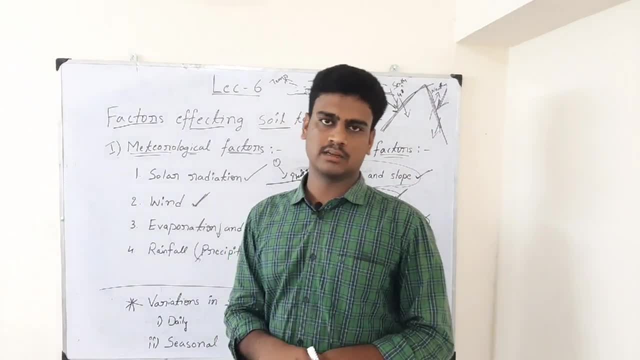 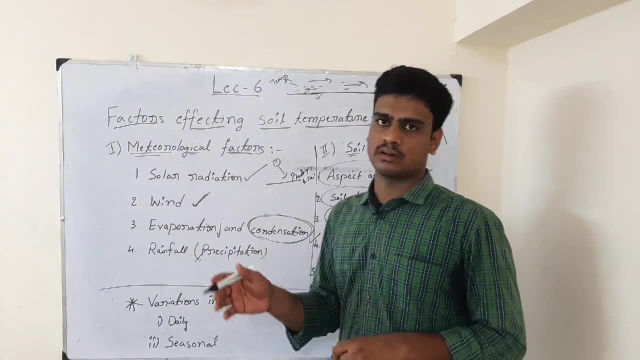 so The meaning of tillage is the mechanical manipulation of soil is called tillage, and tilt means the end product of tillage. That means we are bringing. how can we know the particular soil? Tillage means the tillage means the equal proportion of macro pores and micro pores. 50 percent macro pores should be, 50 percent micro pores should be. So when we have equal proportion, then the soil is well tilled. that we call tilt. When we have 50 percent macro pores, 50 percent micro pores in equal proportion, that we call tilt, The soil is at tilt condition. 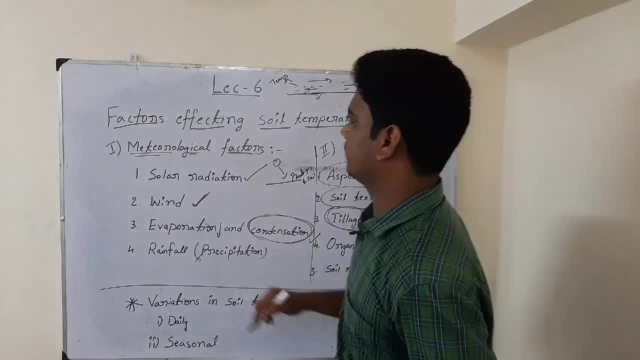 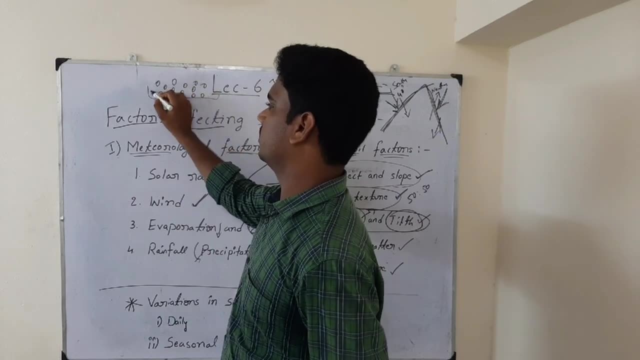 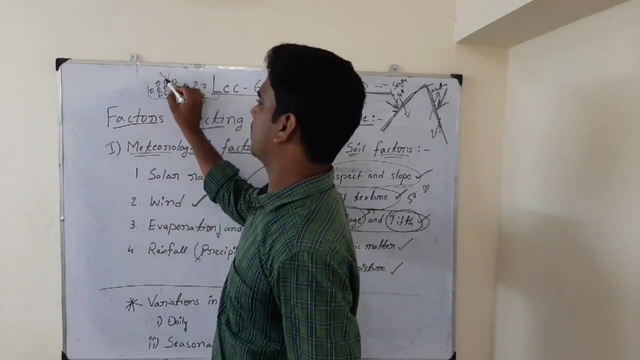 So tillage and tilt, how it affects, For example, after I plough the field, So soil particles are will be get loosened. That is the reason why we are going for ploughing, one of the reason. So when solar radiation comes and hits the soil particle, what will happen? This particular soil? 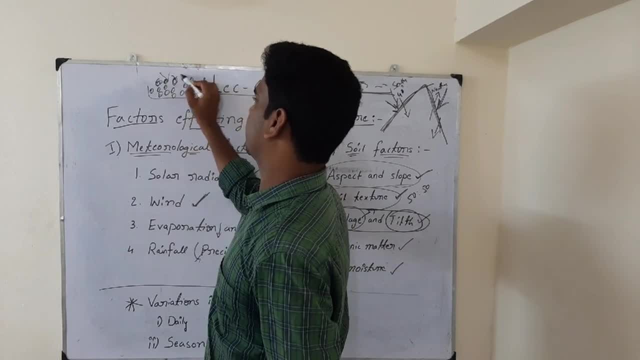 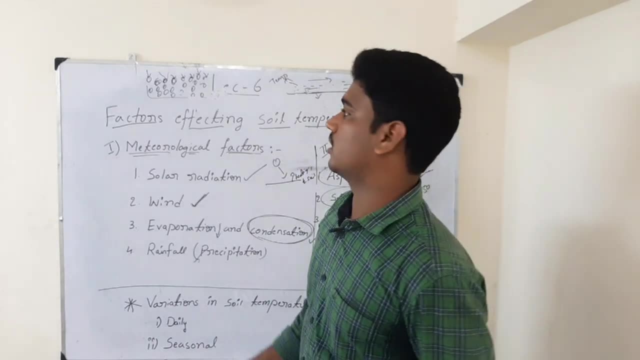 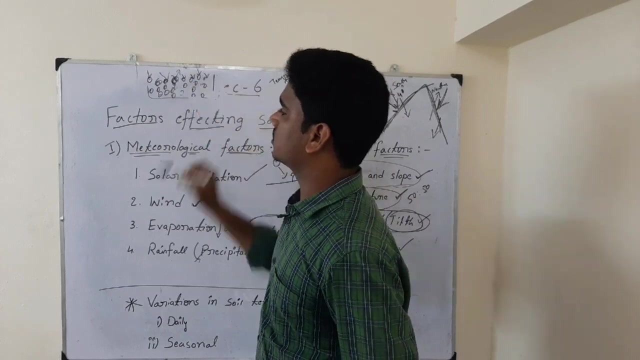 particles will get heats up wherever they are exposing to the sunlight, the particles which all are exposing to the sunlight. But we have loosened the soil already, So this soil particle which got heats up this cannot be transferred into the another soil particle because they are 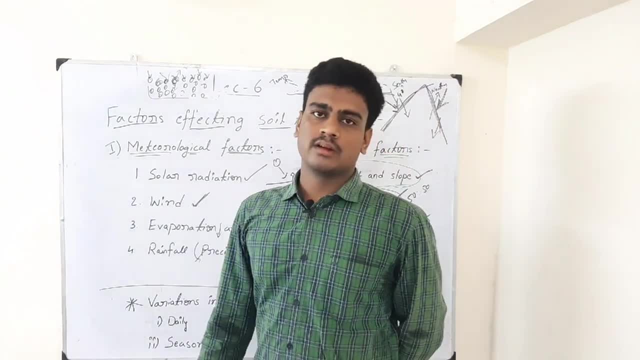 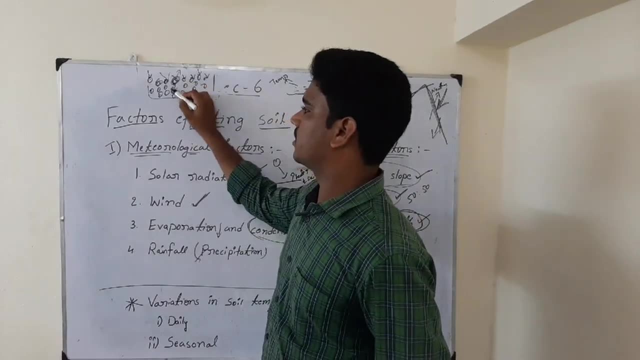 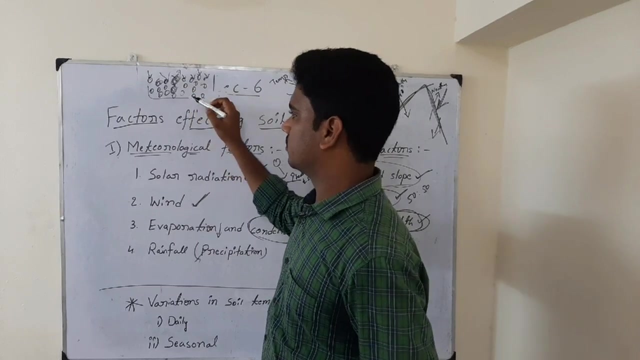 very loose, So condensation. you all know the meaning of conduction, convection and radiation. So here, conduction in conduction. what is the thing? From one material to the other material, by touching, heat, will be transferred. So when the soils are, soil particles are very loose and 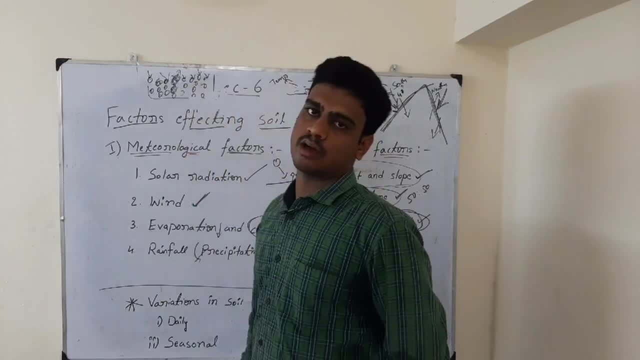 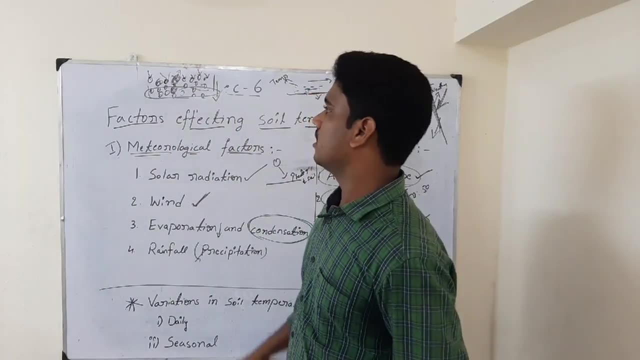 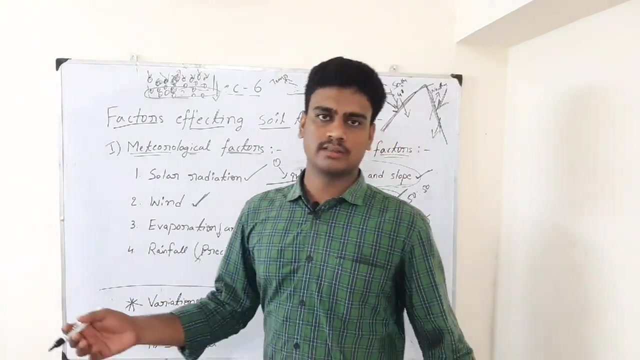 this soil particle cannot transfer the heat into the other soil particle, So the lower depths of the soil particles cannot be heated up well as like uneasiness, until it soil, that means the unplowed soils. there all the soil particles are gathered together and they are very tight in nature. so from the surface of 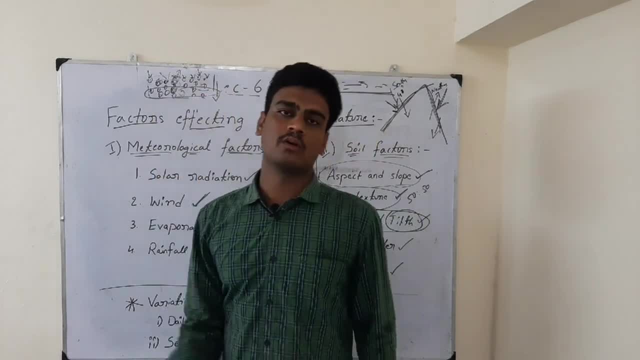 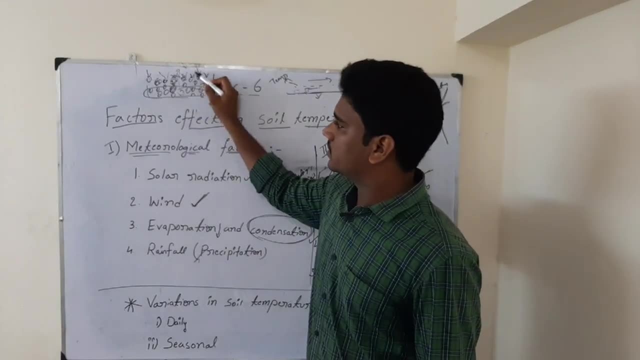 the soil, whatever the heat it is receiving. immediately it can be transferred to the lower depths, but in till it soils are there because of the loosening of soil particles. that temperature cannot be moved into the another, the deeper levels of the soil, because the soil particles are not well. sticked to one another. that is the reason here. the more you go depth to set a depth, the temperature of the soil will be less. but in unplowed soils- any other soil, the more you dig out the soil you feel, the more temperature. that's why the 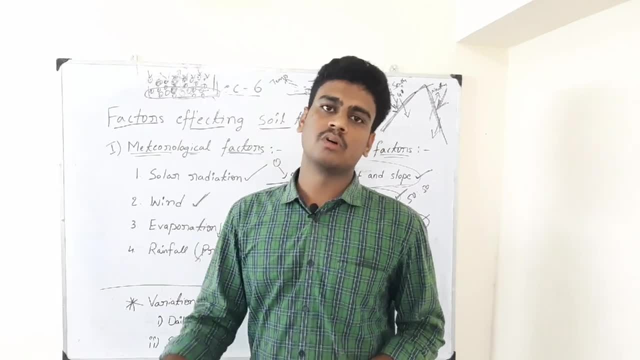 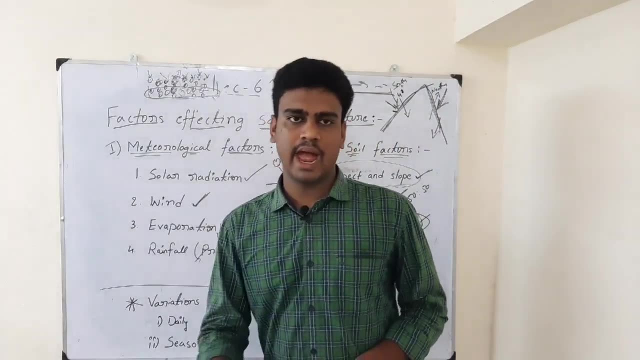 more you dig the pit into the soil that you can feel more warm. then the next one is organic matter. you all know organic matter is in dark in color. when we add much amount of organic matter into the soil it will help the soil to hold more amount of organic matter into the soil and it will help the soil to hold more. 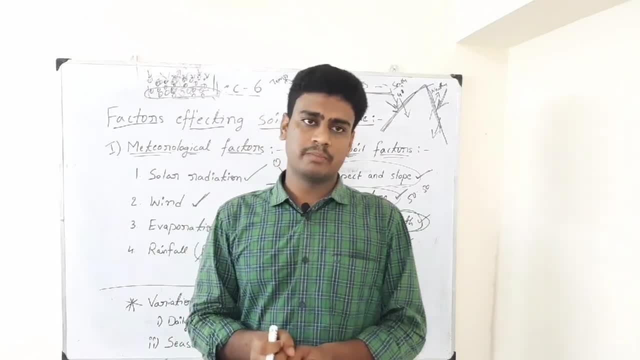 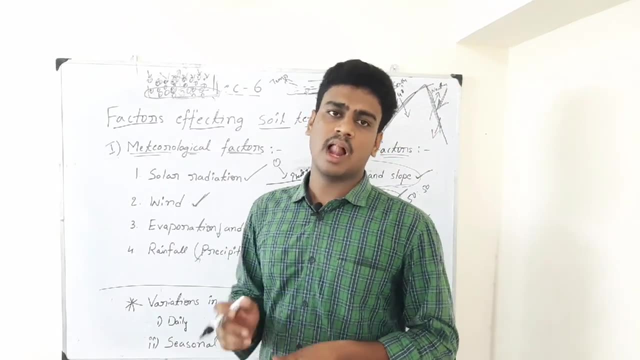 of water. when it holds more amount of water, what will happen? it will maintain the soil temperature. so while it is melting the soil temp, when we have the enough soil moisture in the soil, ultimately it will bring down the temperature of the soil. in that cause, organic matter will help the soil. 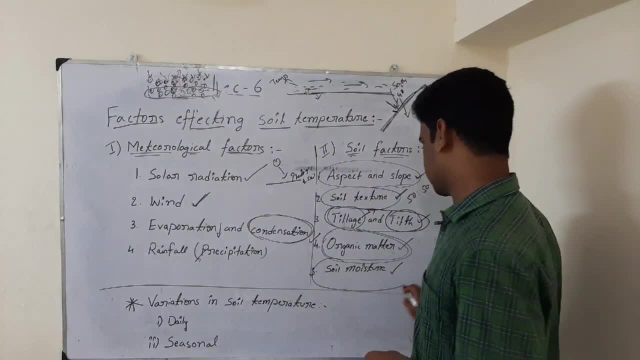 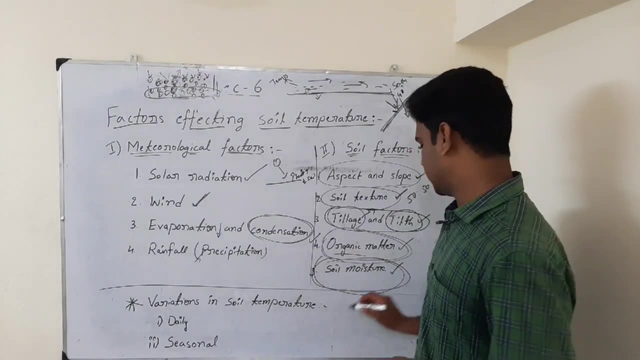 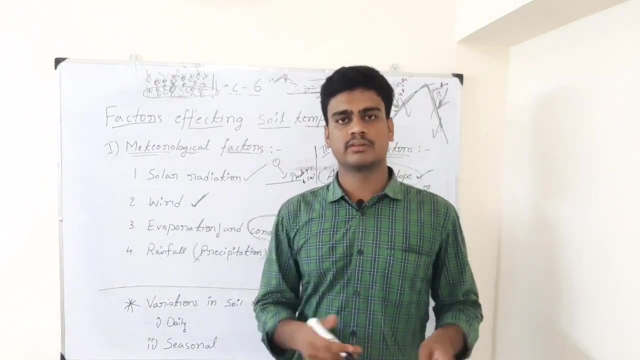 temperature to brings down. then the next one is soil moisture. so soil moisture already in the organic matter I said, when we have more amount of soil moisture in the soil, ultimately it will bring down the temperature of the the soil. But here one thing we have to remember: soil moisture means in what source we are. 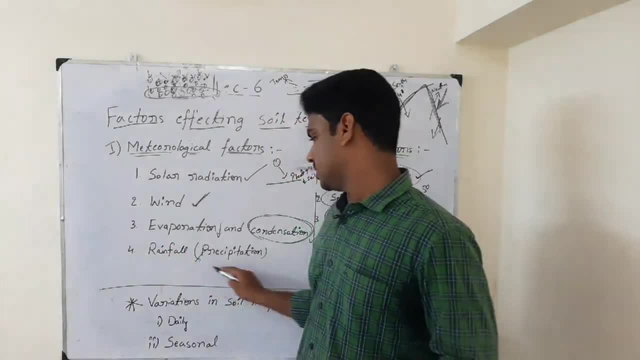 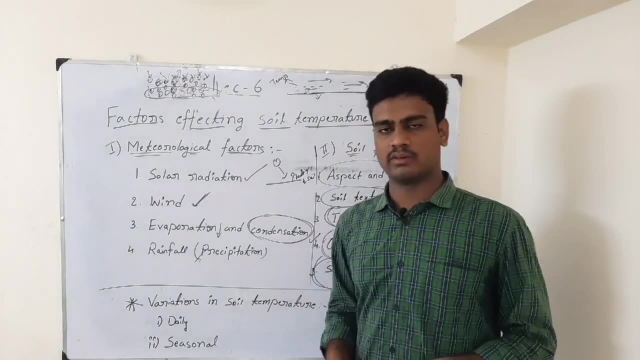 getting that from what source may be. it may be like precipitation, where the temperature of the rain droplet will be depends here in the soil temperature, where if the rain water droplet temperature is high then soil temperature also may be increased If rain water droplet. 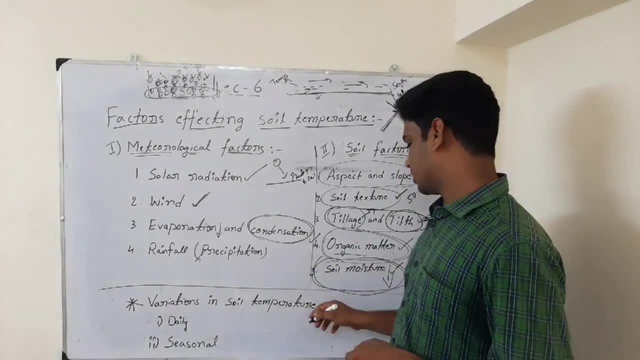 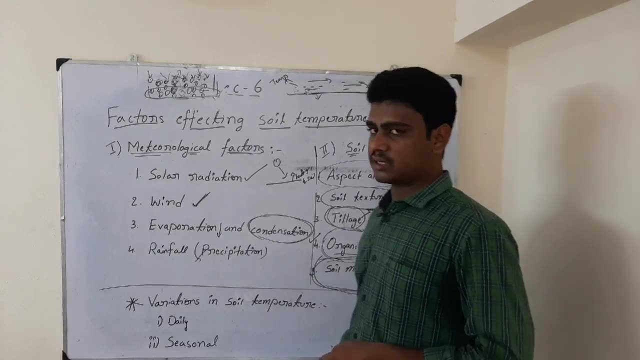 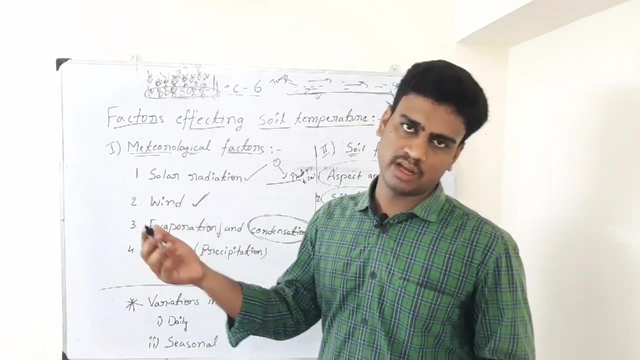 temperature is less, then again soil temperature also can be brought down. So soil moisture plays major role not only in the soil temperature also, and also in plant temperature. When soil moisture is having more temperature, when plant absorb that same moisture, that same temperature will be transformed to the transferred to the plant too. Then the next one is variations. 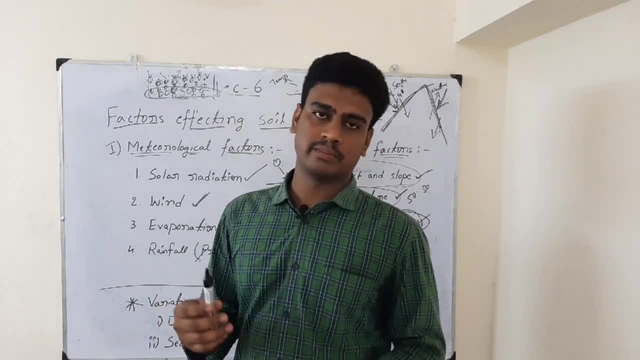 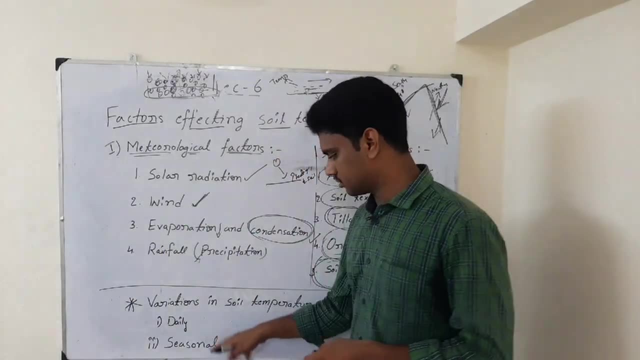 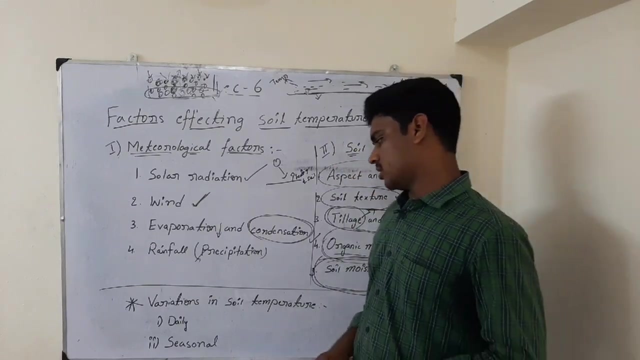 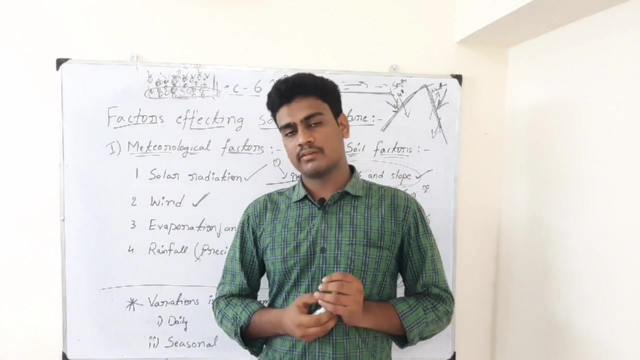 in soil temperature. Already I said variations of air temperature. two types are there: diurnal variation and seasonal variation in air temperature. Same way we are having here also two in soil temperature. So variation in soil temperature and seasonal variations in soil temperature. Dinary variations in soil temperature means, already I said, when soil heats up immediately, when sun rises, and slowly soil also increases its temperature. By the time sun sets, along with that, soil sunset temperature. soil also will be coming down with its own temperature, But it will not maintain the temperature, what it actually got in the afternoon. But when the sun set, is happening along with that. the temperature of the soil also gradually decreases. But during the night time sometimes temperature may be high in some soils, Especially in the deeper layers of the soil. temperature will be varied And also it depends especially on see. I am talking about daily temperature variation, soil temperature variation where we are raising different crops in different fields. 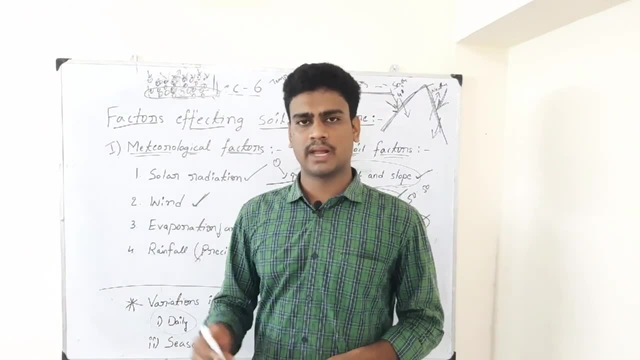 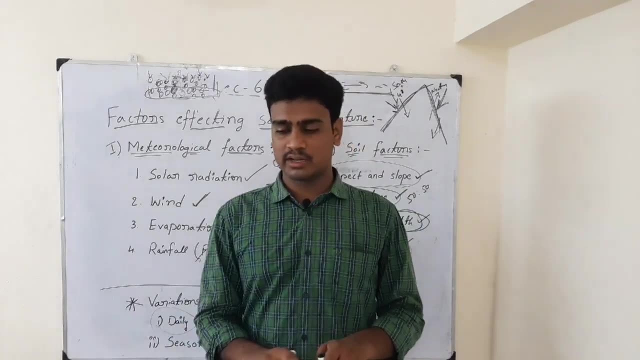 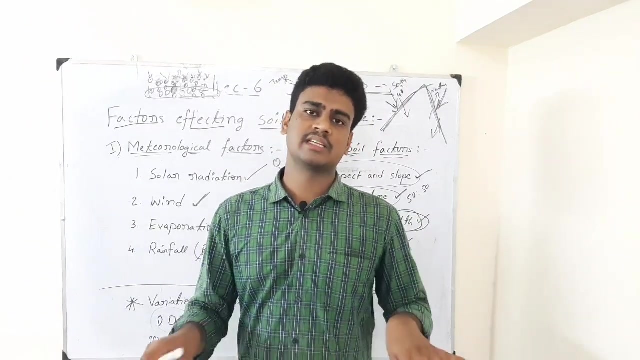 For example, if I am raising close growing crop Like pulses, ground net, any other crop which is growing very close to the soil, those crops will cover the entire land area of the particular field and they will be acting as a mulching and they will be giving the shade effect to the soil, where soil cannot absorb enough solar radiation, which is actually hits the soil. 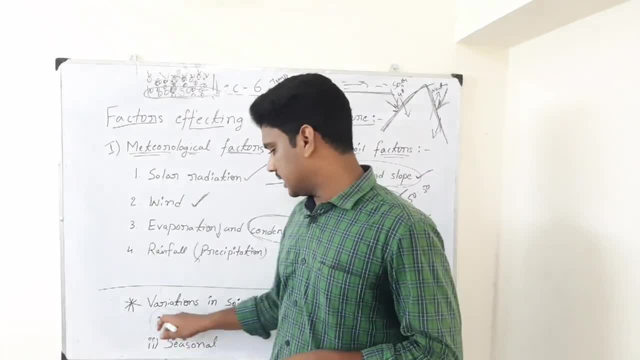 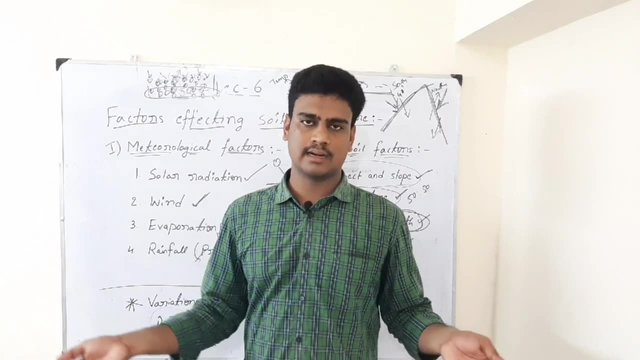 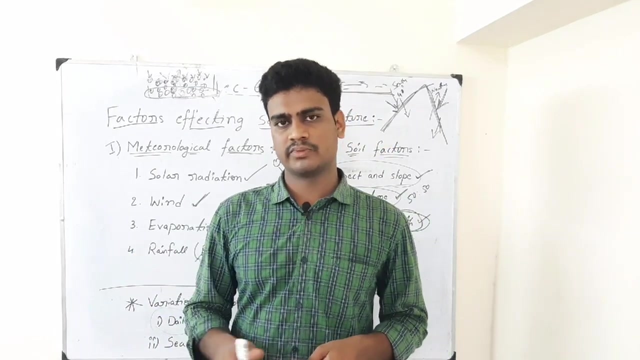 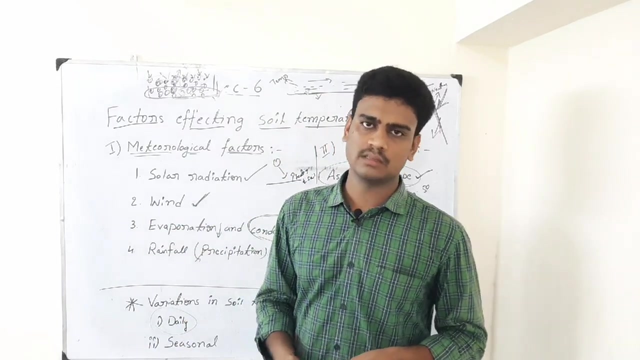 So that is where crop reduces the soil temperature. So daily temperature will be varied as such. But if some crops will be there where they are very broad, Broad space, like cotton and maize or sorghum, which are little broaded spaced crops- broad spaced crops where temperature raises and when solar radiation is high. some amount of solar radiation can easily hit directly into the ground and temperature can be increased. So, likewise, daily temperature will change based on the crop And also, not only that, based on the day time and night time, in particular, during summer season, again, temperature will be varied. During winter season, temperature will be there Varied that we discuss in seasonal soil temperature variation. 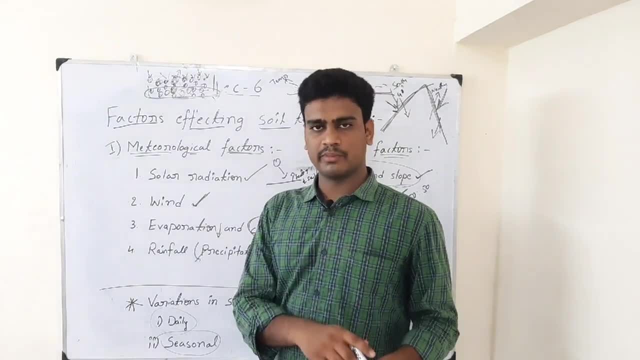 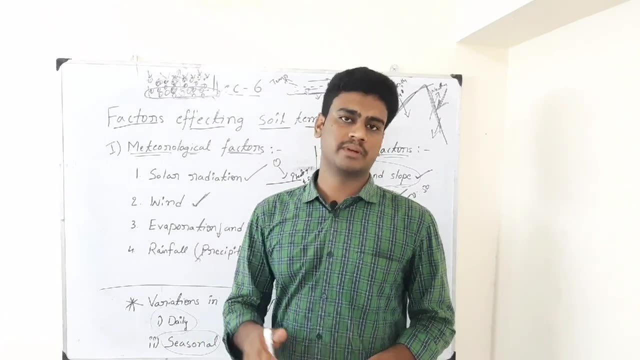 So in daily temperature variation from the crop to crop it will be varied, And also from soil to soil it will be varied. And also in that particular day how much temperature actually given into the soil from the sun, that also will be different. So every day variation, we find One maximum temperature and one minimum soil temperature. This soil temperature we measure by using the instrument called soil thermometer. we will be having three types of thermometers based on the depth, not only three. how much depth you want, you can have that. accordingly, you can insert the soil thermometer into the. 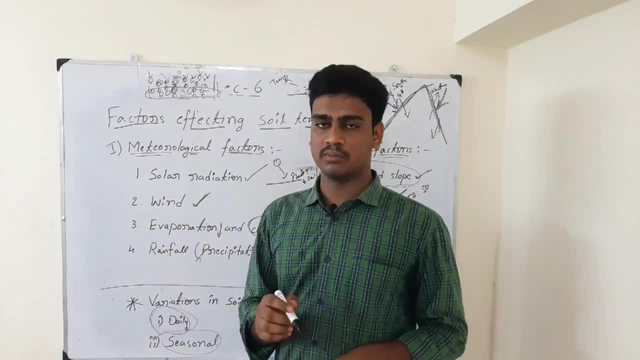 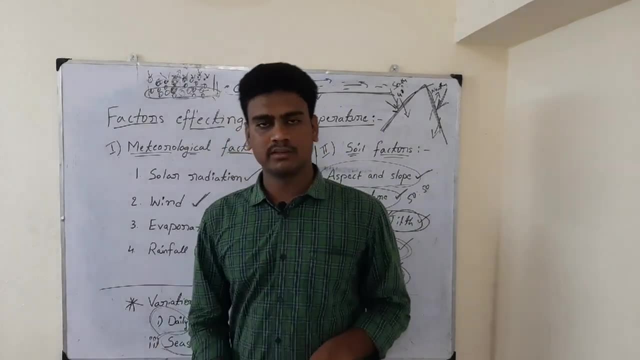 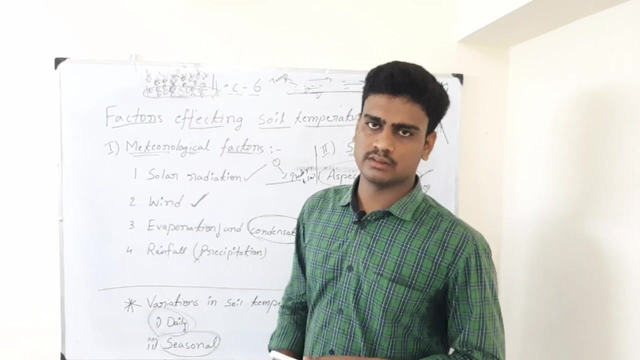 soil and we can get the temperature of the soil. so soil thermometer is the instrument that we use to measure soil temperature. then the next one is seasonal variation: meaning of seasonal variation. we all know that the air temperature, what we studied, same thing here, also to be based on the season- soil temperature will be varied during the winter season soil. heats up slowly because of the less incoming solar radiation temperature, and during summer season incoming solar radiation power is high. so in during summer season soil temperature will be little high. but in rainy season soil temperature will be less because often we get rains and the drain water will bring down the temperature of the soil. but though 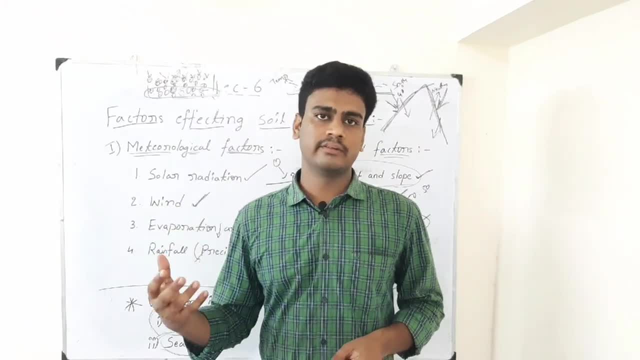 Sometimes our soil temperature will be slightly above that temperature, as you can see the arrangements between the soil temperature. so we have to check one or two times per day, so any certain duration we have to check the water temperature, also based on times. rain may not happen, but still the rain moisture whatever the rain comes, so far that 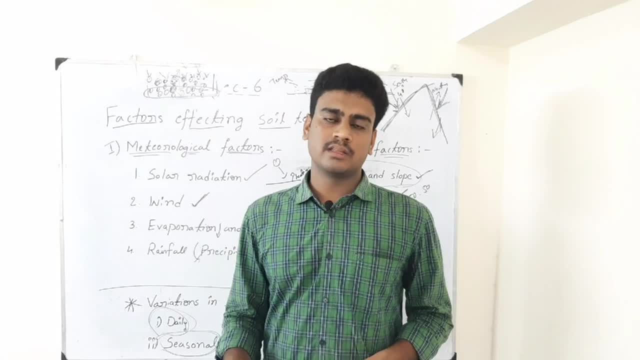 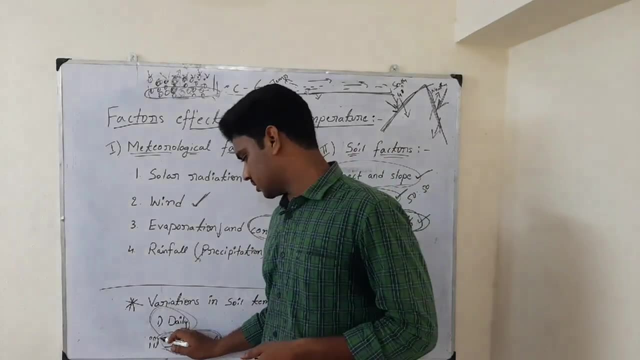 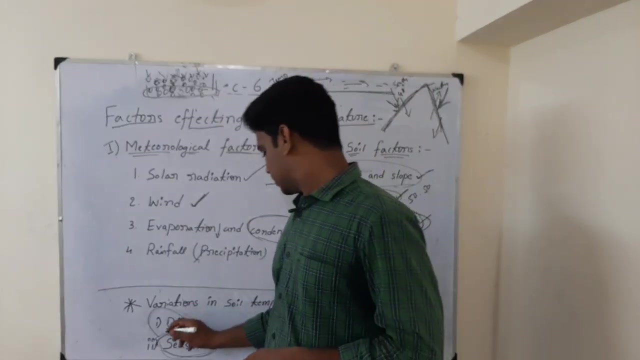 moisture will be remained in the soil. that will remain the soil temperature as such. sometimes it may rise, but again, when rain comes again, it will fall down. so seasonal temperature variation also will be there because of different temperatures. so this, these are the things which we have to. 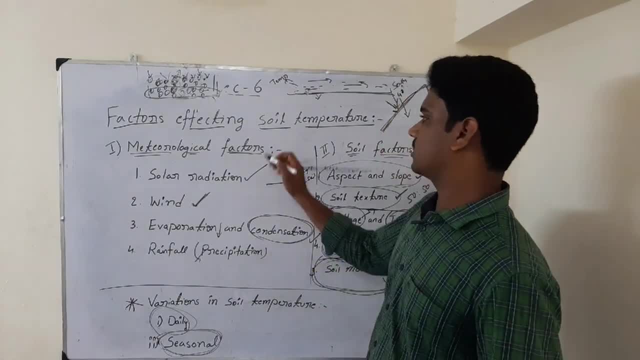 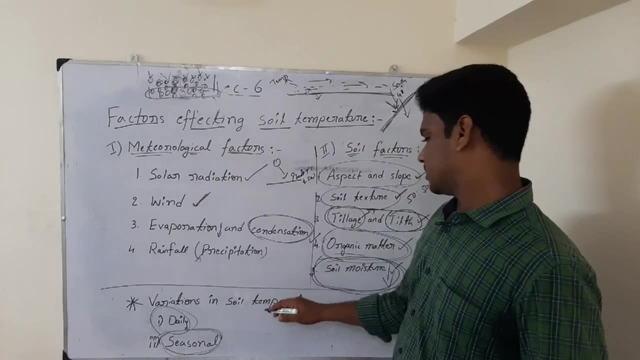 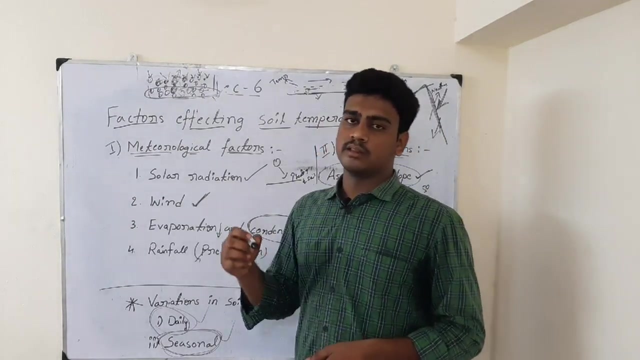 discuss in the soil temperature. so in this lecture we have seen factors which are affecting soil temperature, from which meteorological factors and soil factors. apart from that, we have seen variations in soil temperature. first one is daily variation. second one is seasonal variation. in the last class we have seen the importance of soil temperature. so these are the things we have to. learn from soil temperature. thank you, 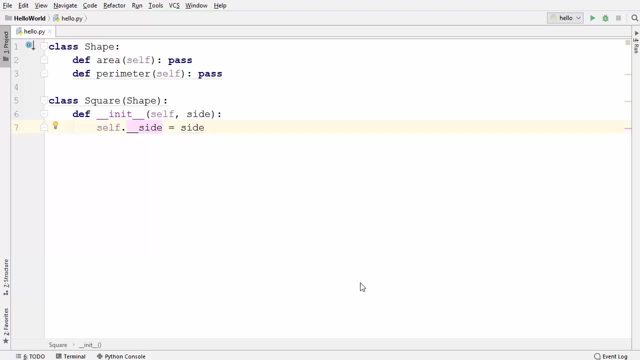 In this video, we will talk about creating abstract classes in Python, So let's get started. So, to start with, I have here two classes. One is a shape class and other is a square class. In shape class, I have two empty methods- One is area and other is parameter- And I am using shape as a super class and square as a sub class, And square class is inheriting from the shape class.